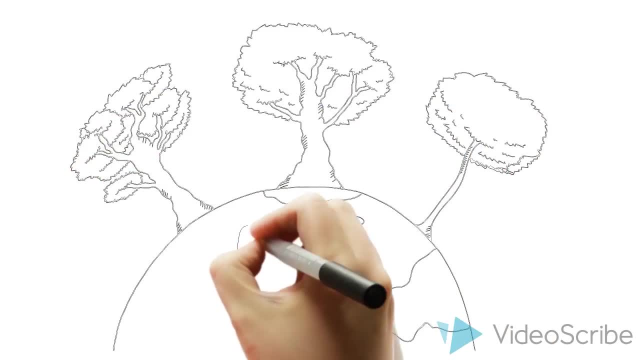 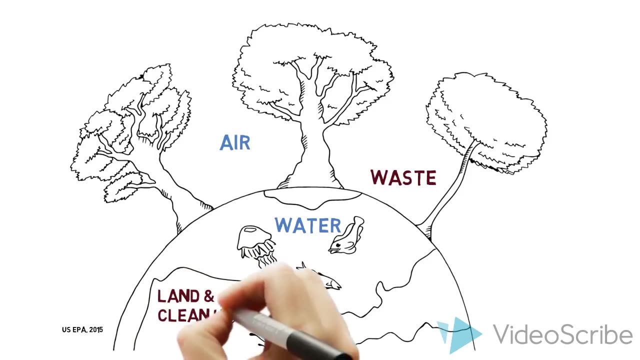 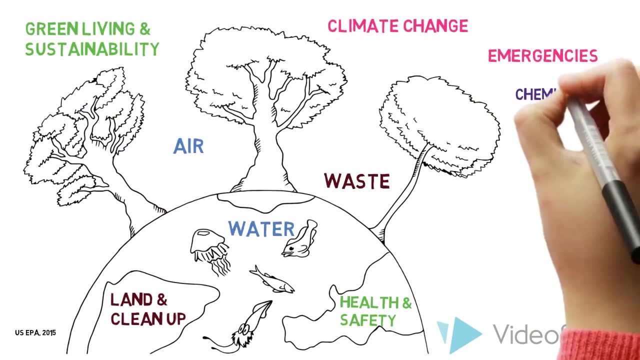 The United States Environmental Protection Agency has identified ten issues of concern in this matter: Air, water, waste, land and cleanup, health and safety, climate change, green living and sustainability, emergencies, chemicals and toxins and pesticides and agriculture. By focusing on these issues, environmental engineers improve and maintain the environment for the protection of human health and ecosystems. 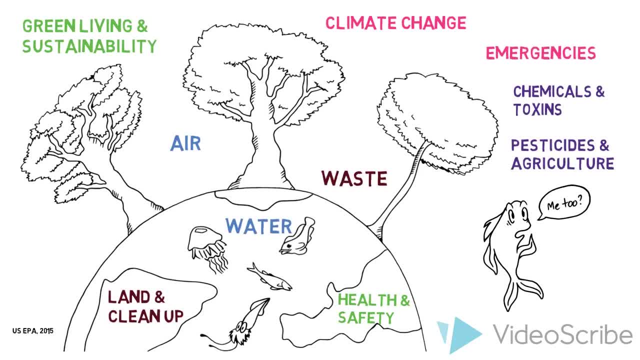 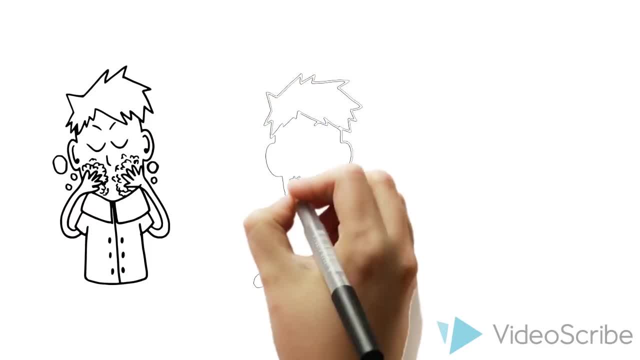 Me too, Yes, you- To see how important environmental engineers are to our life. let's look at our own daily routine. When you wake up in the morning, what is the first thing you do? You wash your face, brush your teeth and you use the restroom. 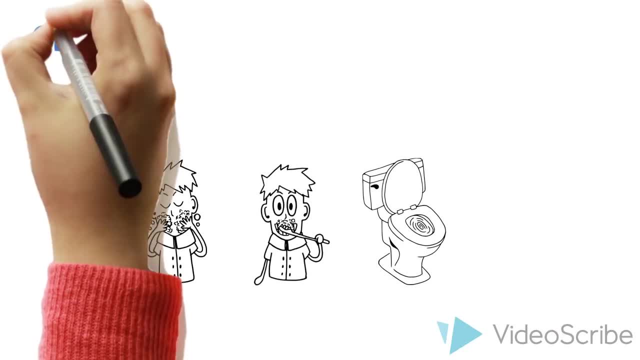 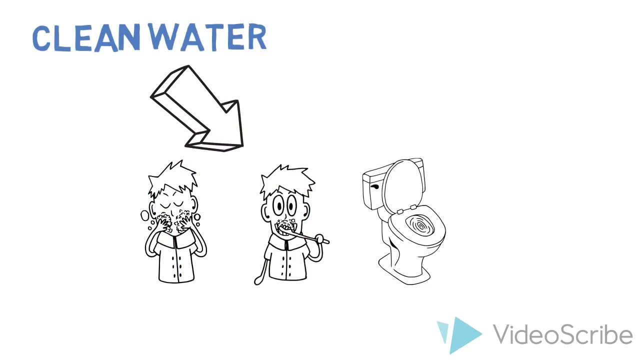 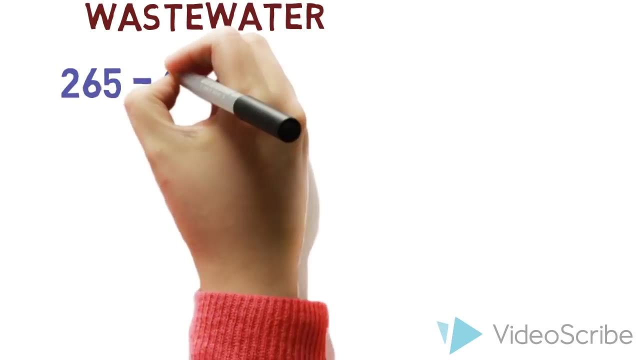 To do all of these activities, you need clean water, Environmental engineers, clean river water and groundwater to provide you with safe drinking water which you use for all your activities throughout the day. What happens to that water that you use? In a day, each of us generates 265 to 375 liters of wastewater. 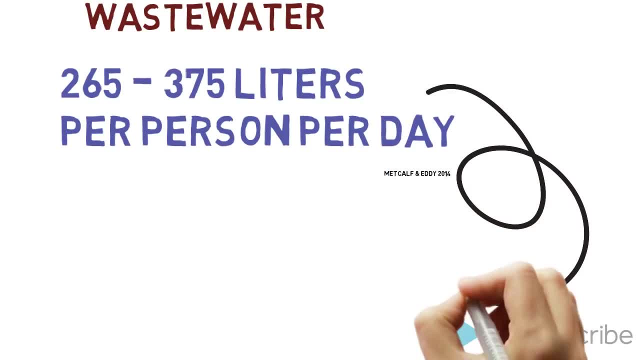 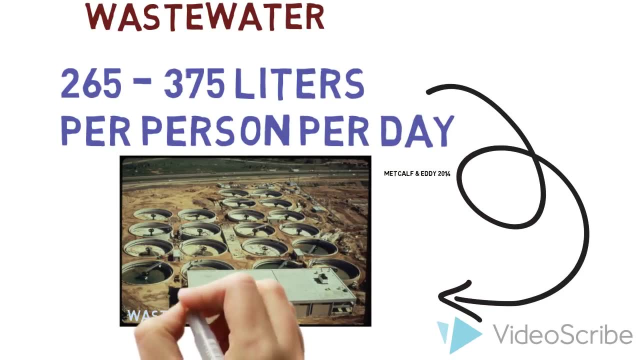 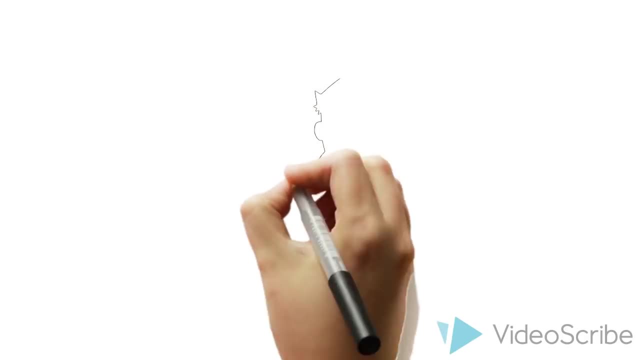 All of that has to go somewhere right. All this wastewater is sent to treatment plants near your house. Environmental engineers design these plants to clean millions of gallons of water each day in order to maintain water quality of rivers and oceans. Moving on, Now that you're dressed to go to school, you go to the kitchen and eat breakfast. 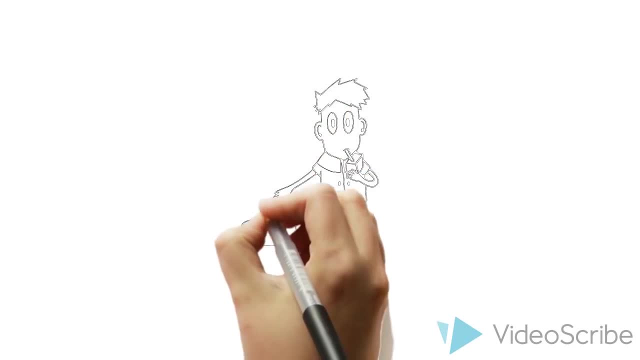 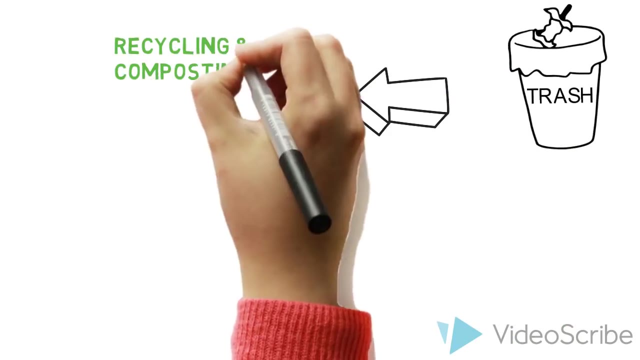 You throw away any leftovers and trash Cereal boxes, wrappers, paper towels. Where does it all go? The trash you generate is collected from your house and is either recycled, composted, incinerated or buried in the landfills. 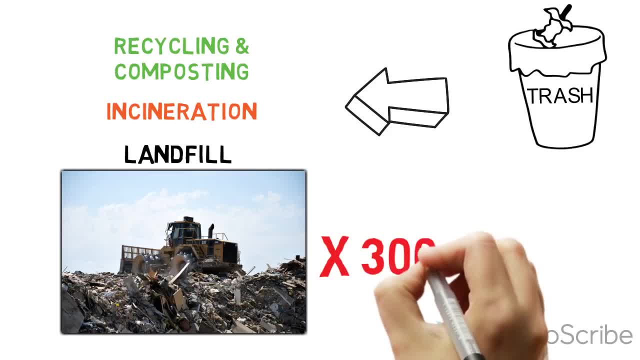 There are more than 3,000 landfills in the United States that are specially engineered to hold tons of solid and hazardous waste generated by people and industries, so that toxic chemicals in the waste do not pollute the soil. Okay, let's go back to your morning routine one last time. 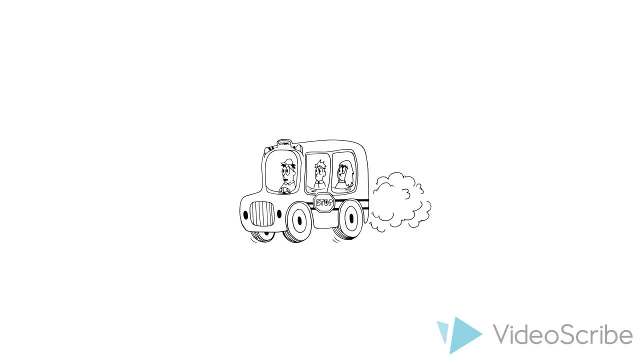 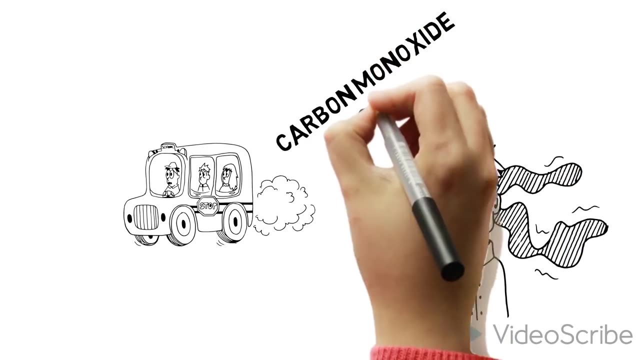 You've finished breakfast and you're ready for school, You get on the school bus. You may have noticed that buses spit out smoke when they run. sometimes The smoke contains gases such as carbon monoxide, carbon dioxide, which deteriorate air quality.